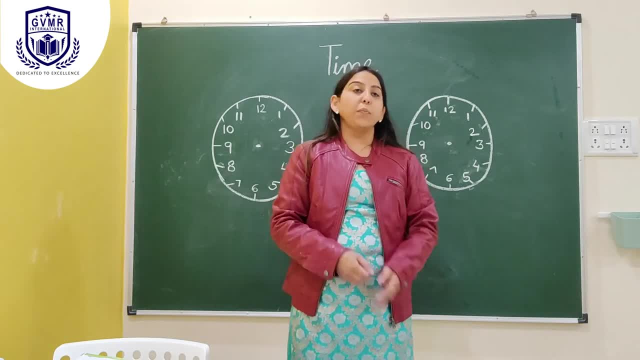 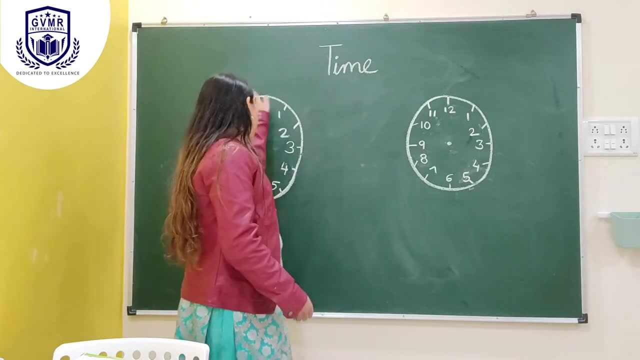 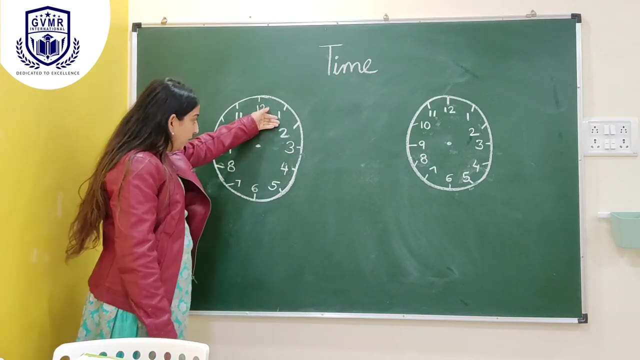 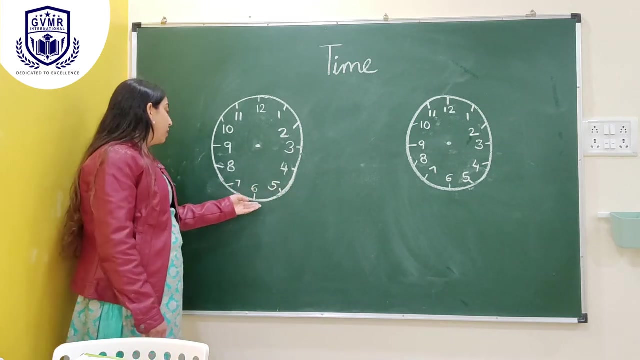 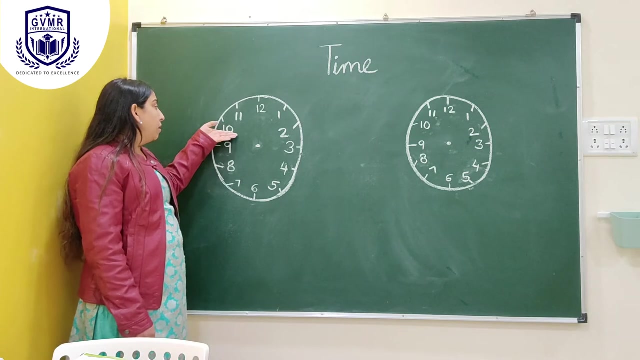 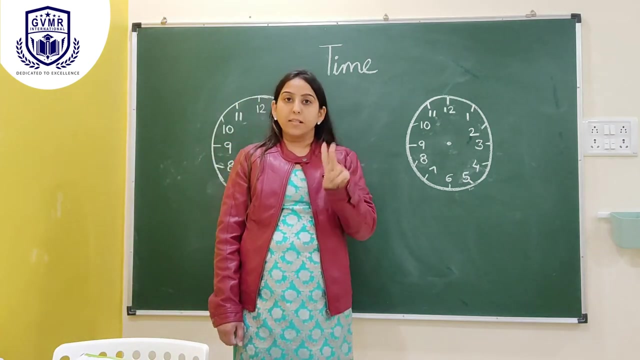 Good morning children. Today we are going to study the concept of time. A clock tells us the time. The face of the clock has 12 numbers. How many numbers are there in a clock? face 12.. 1,, 2,, 3,, 4,, 5,, 6,, 7,, 8,, 9,, 10,, 11,, 12.. It has two hands, One short and one long. How many hands are there in a clock? Two hands? 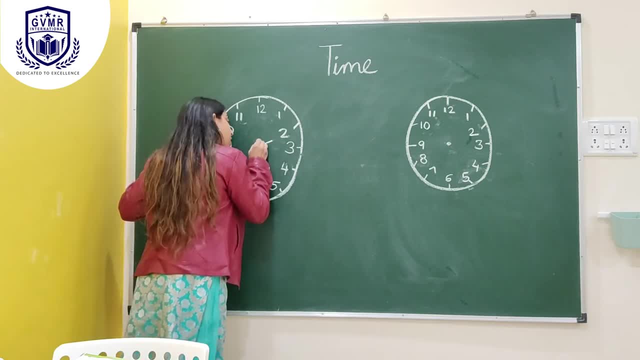 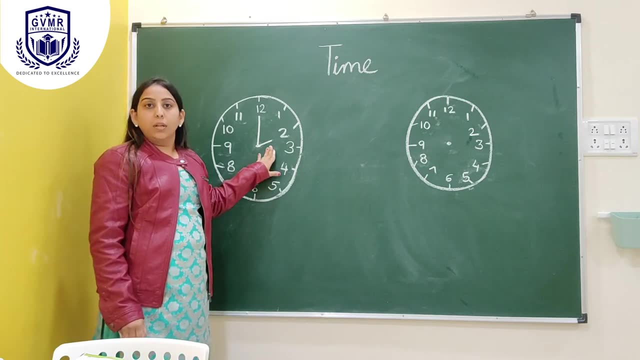 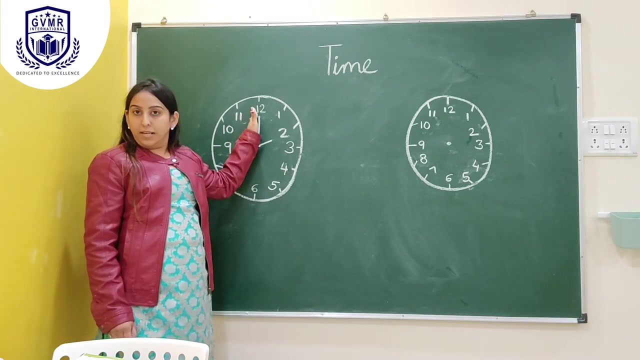 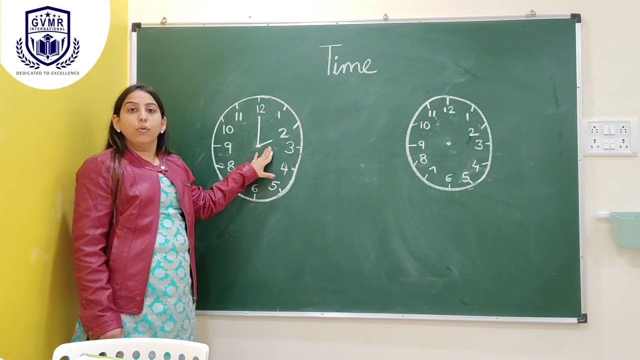 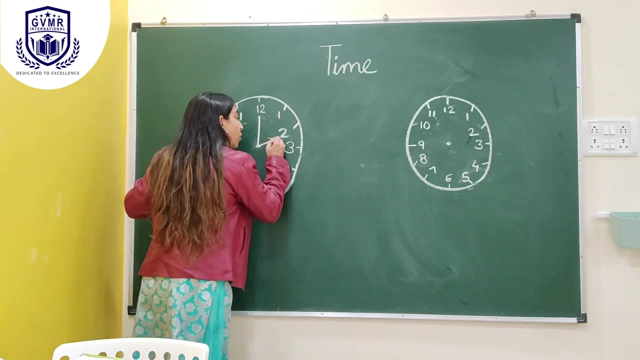 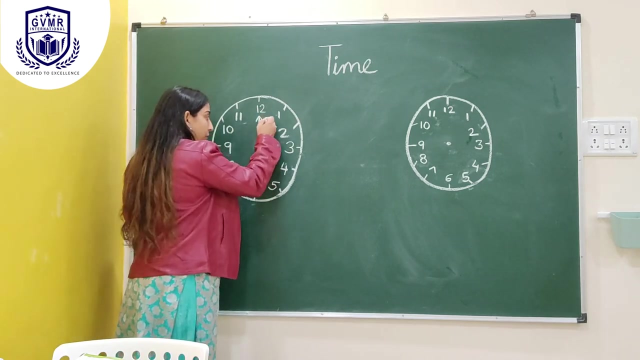 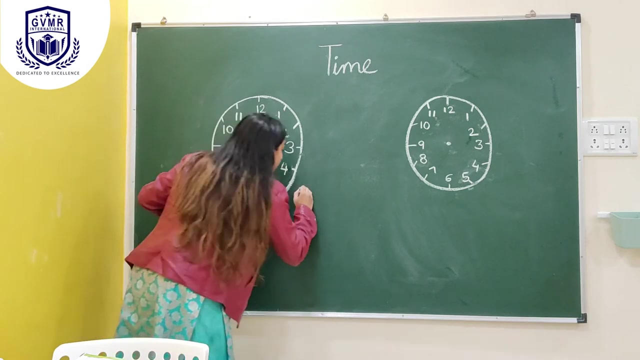 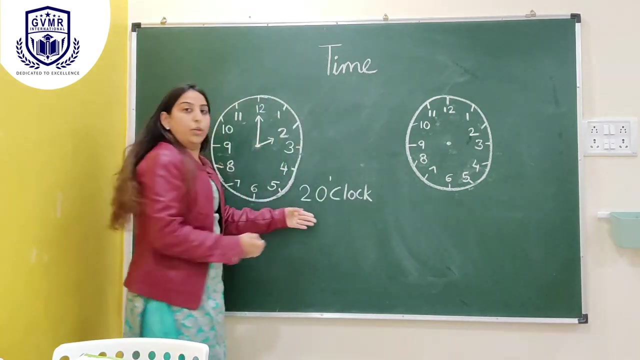 One short, One short and one long. The shorthand shows the hours, The shorthand shows the hours and the longhand shows the minutes. In this clock, the shorthand points to 2.. In this clock, the shorthand points to 2.. And the longhand points to 12.. The longhand points to 12.. So the time is 2 o'clock. The time is 2 o'clock. 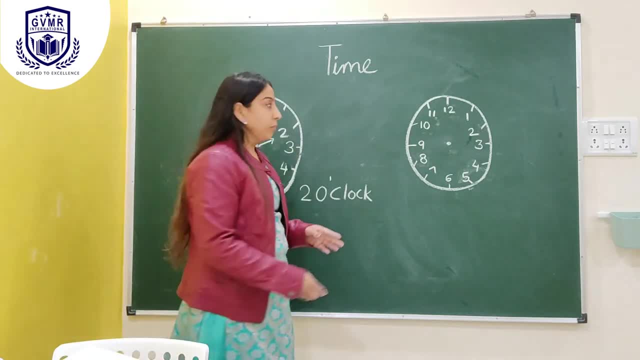 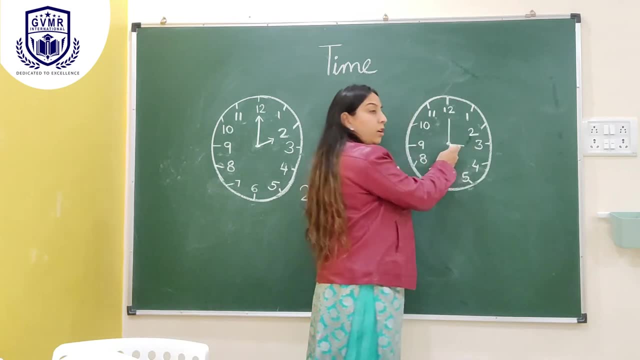 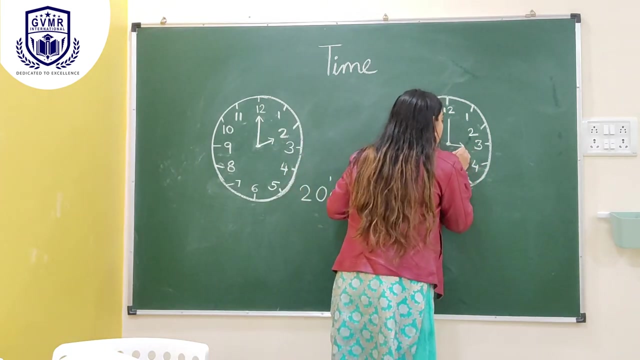 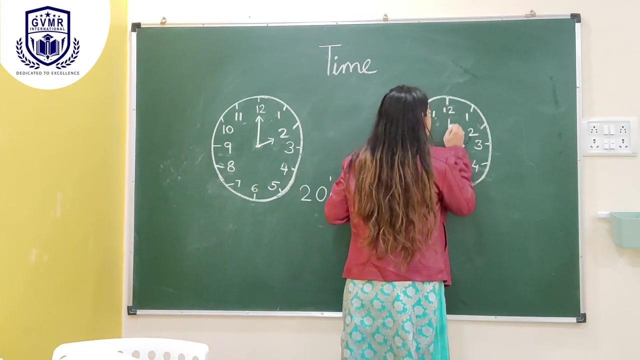 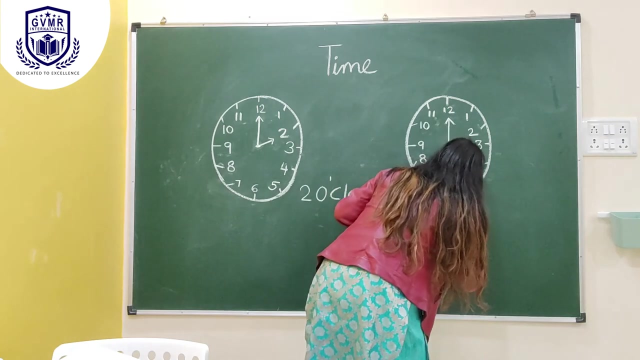 Now let's do one more example. Two hands are there, One long and one short. The shorthand points to number 3.. And the longhand points to number 12.. It means the time is 3 o'clock. Two hands are there, One long and one short. The shorthand points to number 3.. 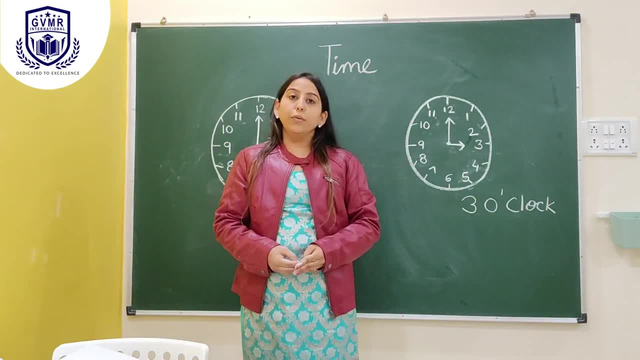